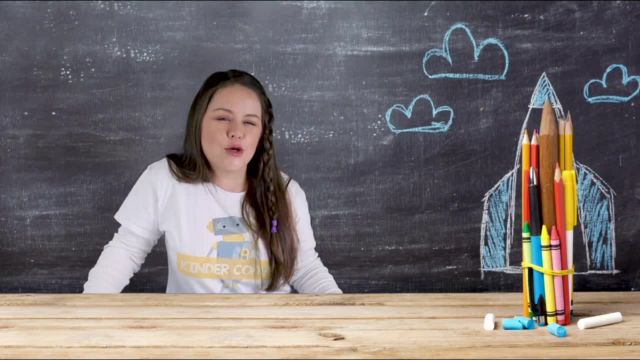 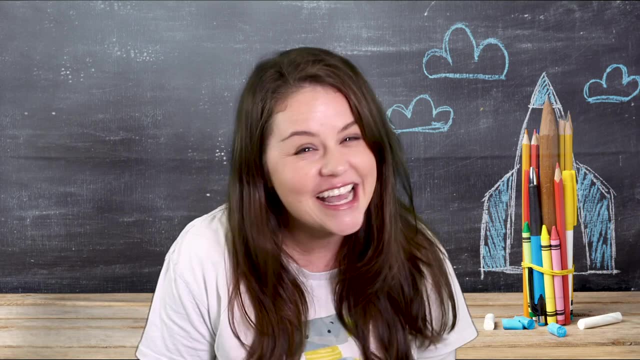 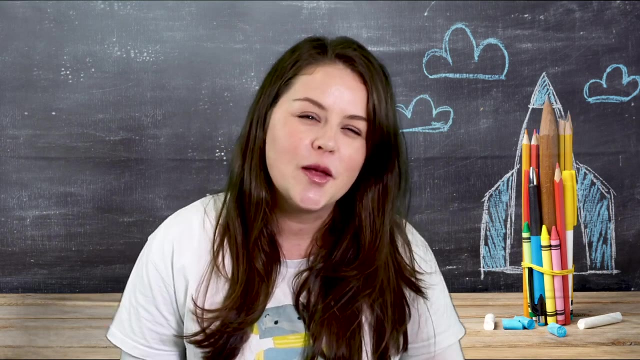 Hey, it's Lisa here from Happy Explorers, and today we're going to talk about kindergarten robotics. So you're going to introduce kindergarten robotics into your classroom- Excellent, Good job. So kindergarten robotics is all about learning what a robot is and how we talk to robots to get them. 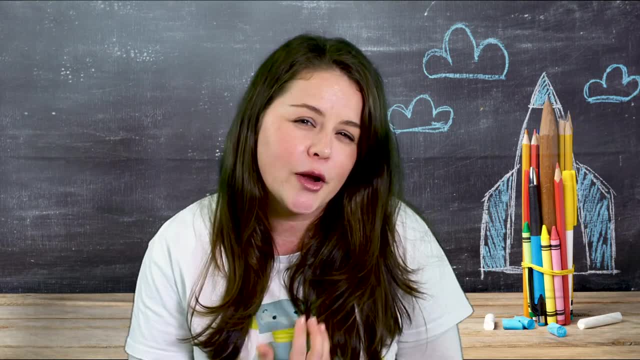 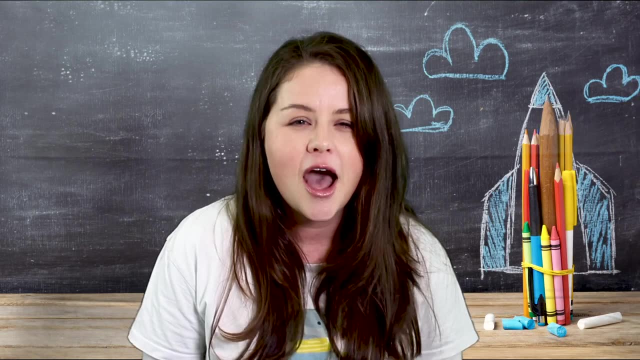 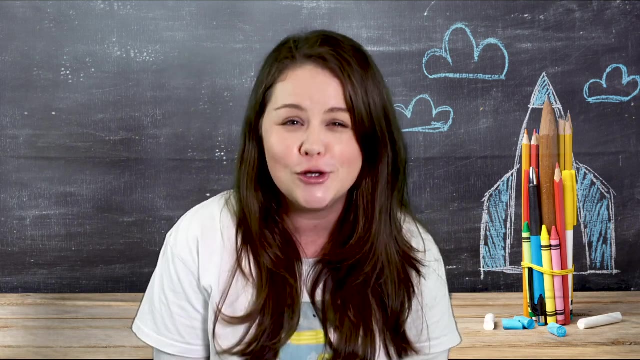 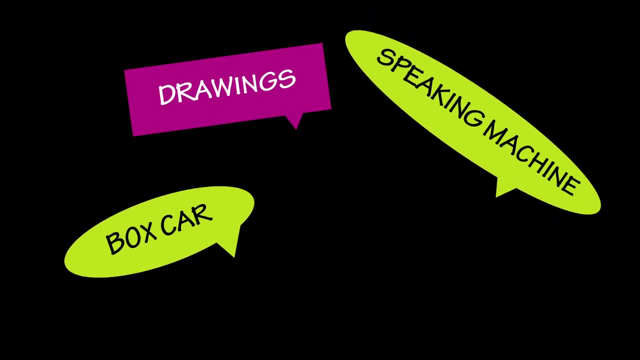 to do the things that we want them to do. Now, kindergarten robotics is totally play-based, And in this video, I'm going to teach you in five simple steps how you can introduce robots into your classroom. What's a robot- Information- What's a robot- History. A robot is a computer and a machine put together. 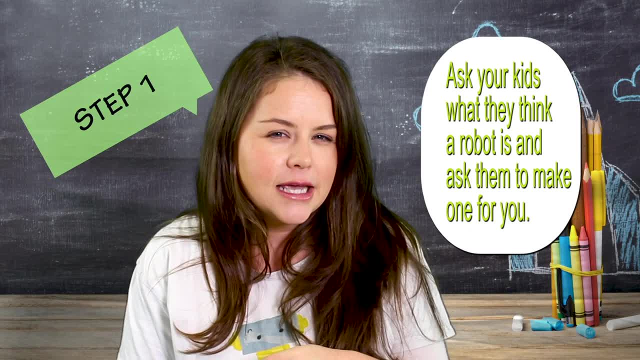 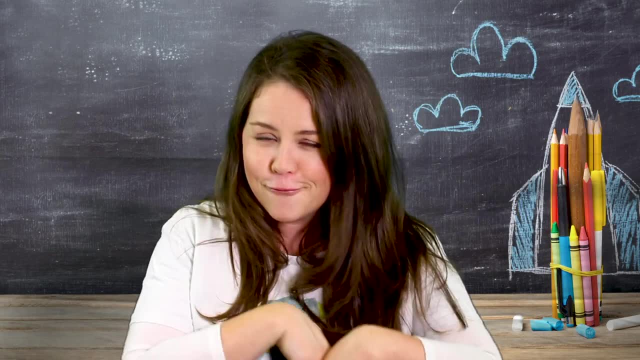 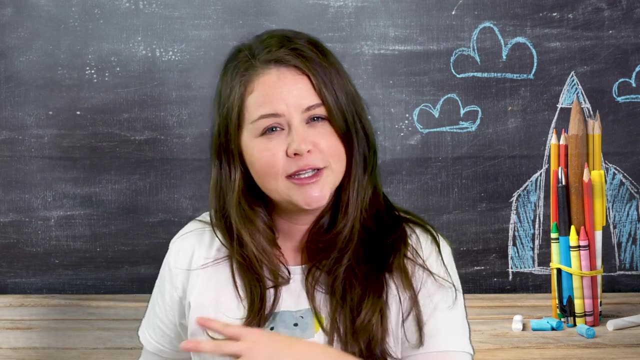 So how I like to introduce robots to my kindergarten kids is I get them to make a robot. I get them to make play-doh robots. Now, no rules apply here and they can create whatever they like. The most important thing in this part is opening up conversations about robots being machines. 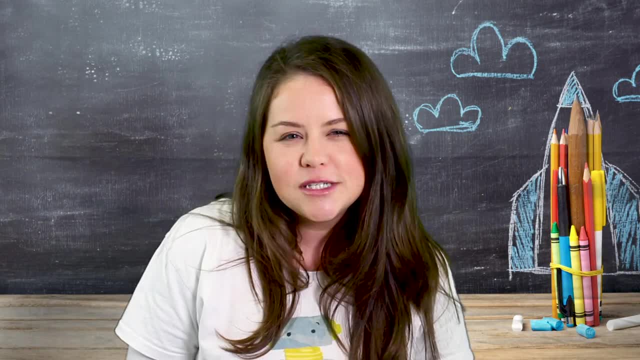 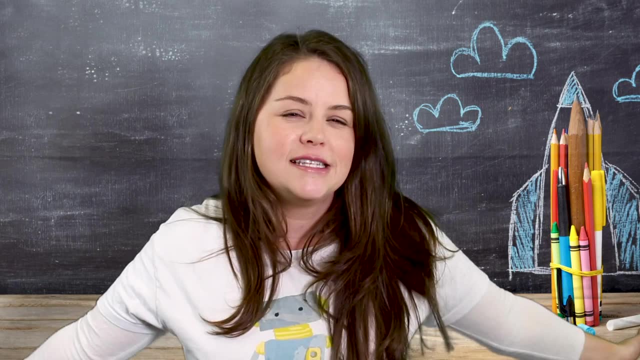 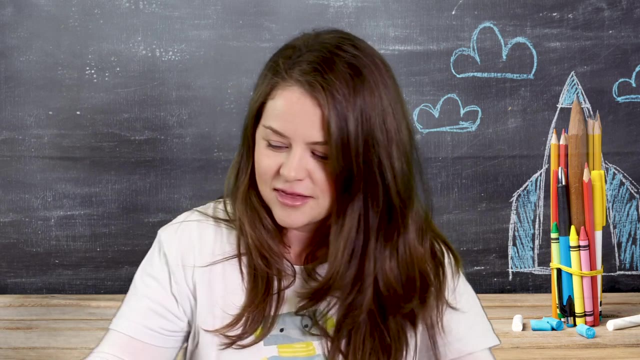 being part computer and also getting them to think about what their robot might be able to do. Now I've seen heaps of crazy stuff and I love it, So here's some examples of perfect little robots. So once you've introduced robots into your classroom and seen what the kids 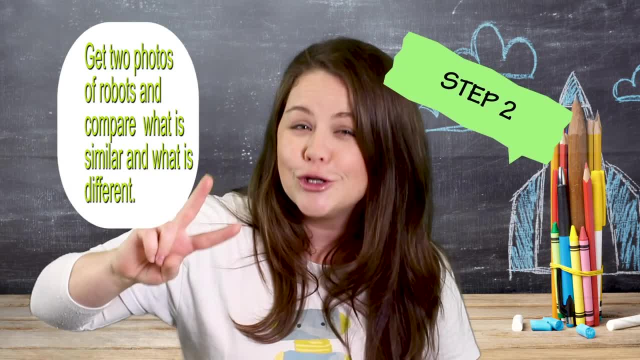 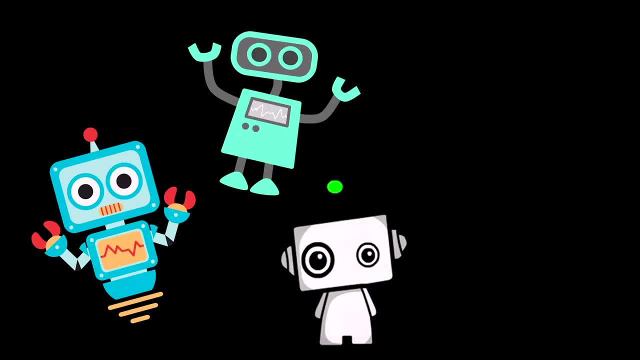 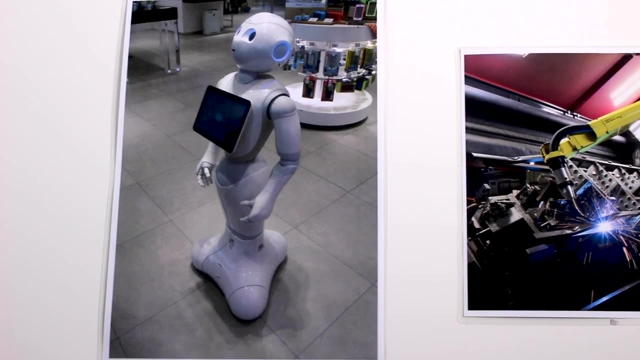 like and know about them. then you can move on to step two, which is all about comparing robots. Robots come in all different sizes and shapes, and it's a really good activity to compare two different photos of robots. In this classroom activity, we're going to print off different photos. 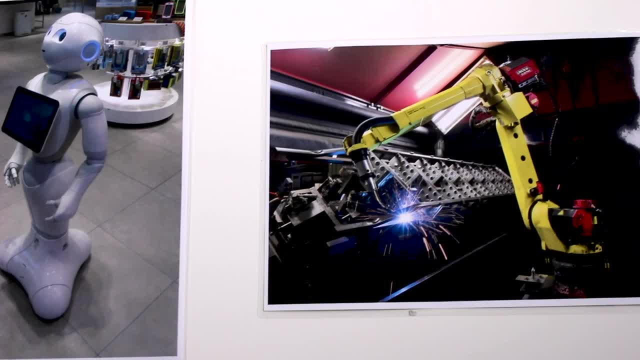 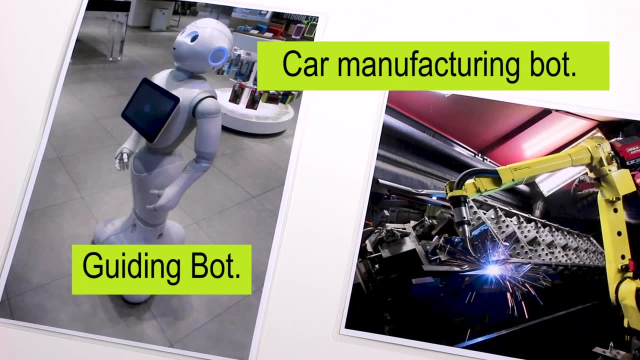 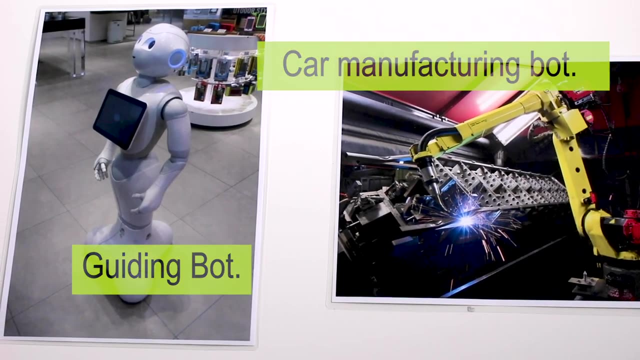 of robots and then ask the kids to tell us which one they think the robot is. Now, they always recognise the humanoid bot, but they cannot understand that the other one is a robot. The most important thing in this activity is allowing the children to explore. 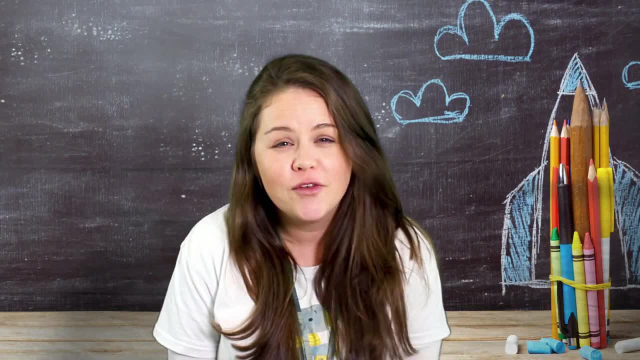 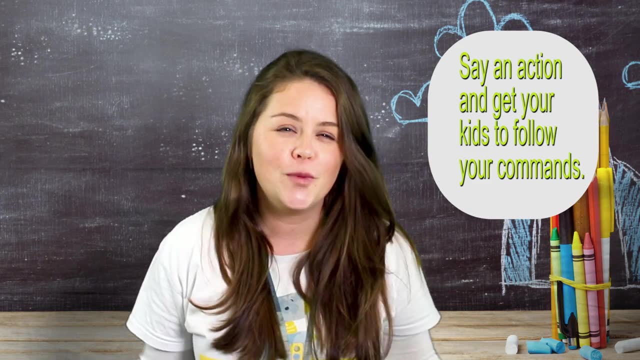 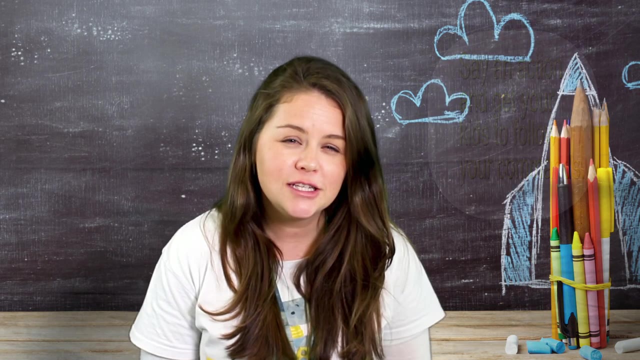 the similarities between the two different pictures. I'm moving on to step three, and step three is a verbal coding challenge, And this is cool because it helps children understand that robots follow commands. So what What you need to do for this activity is tell your class that they are now robots. 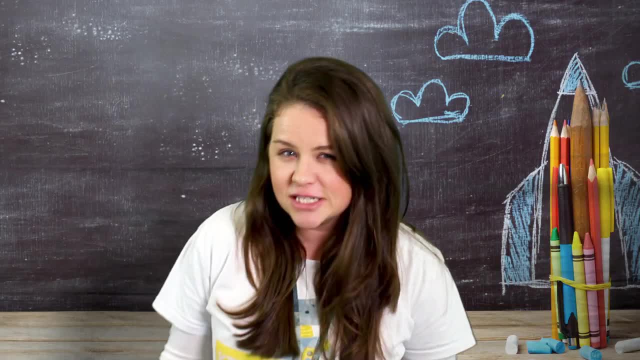 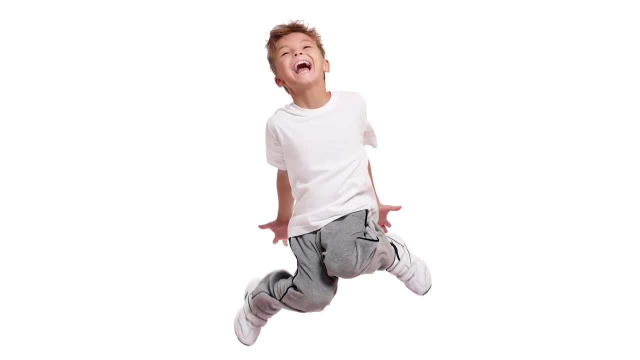 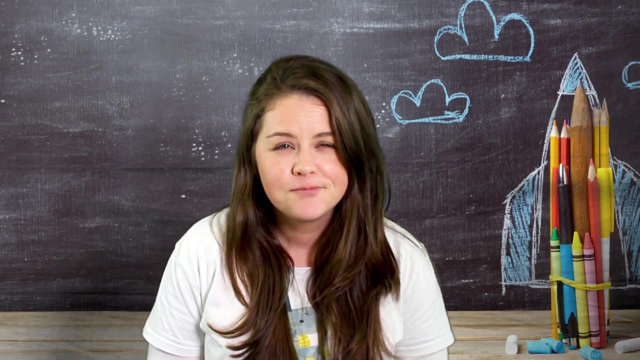 and they have to follow your commands. Then you are gonna say actions like: step forward, step backwards, spin right, spin left, jump up, sit down, clap your hands, balance on one leg, pick up an object. laugh, that's a great one. 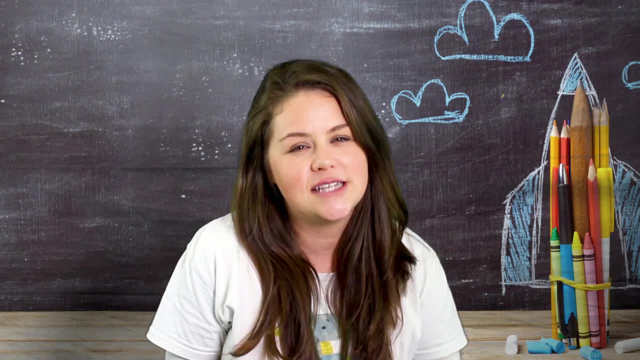 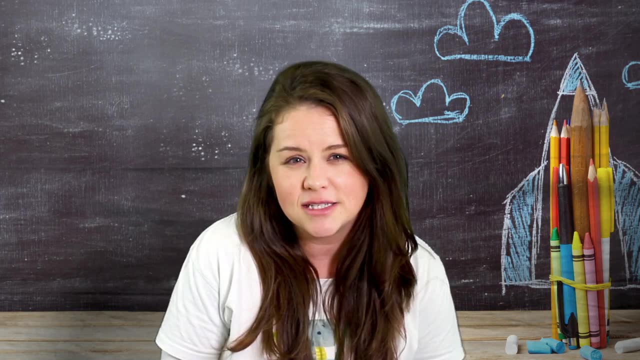 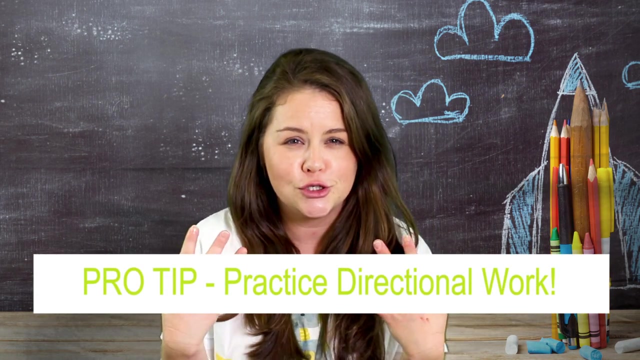 So the main thing in this activity is to get your kids to understand that robots can't think for themselves. They need you or a coder or something else to tell them what to do. So here's a pro tip for you Now, if you're going to be looking to introduce robotic toys: 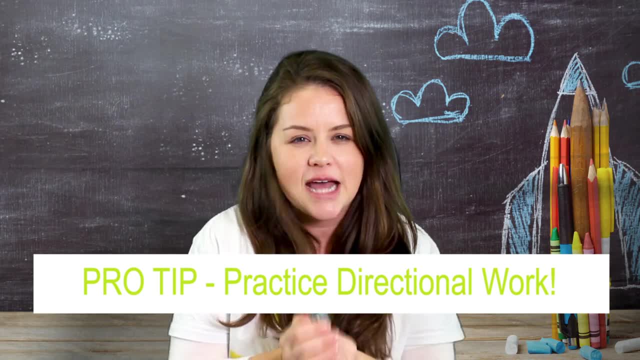 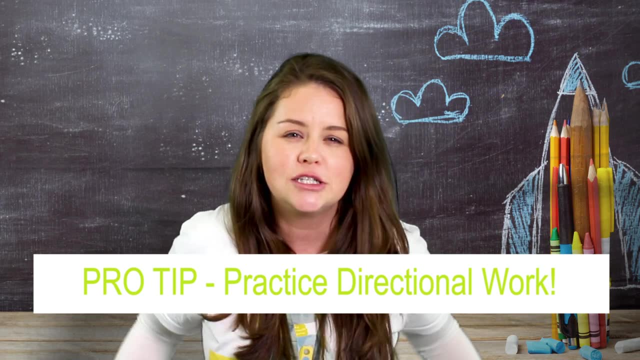 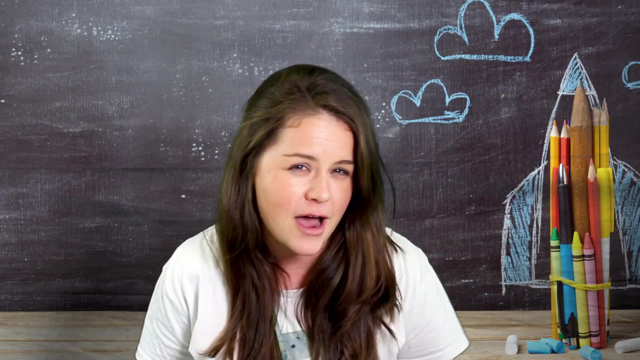 in the future into your classroom, then definitely start working on teaching your kindergarten kids left and right. It's a really basic concept, but you do need to scaffold that knowledge over time because all coding toys tend to use left and right as a way to code the little robots in those kids. 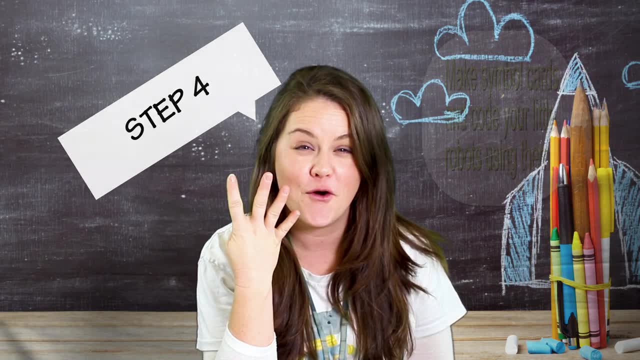 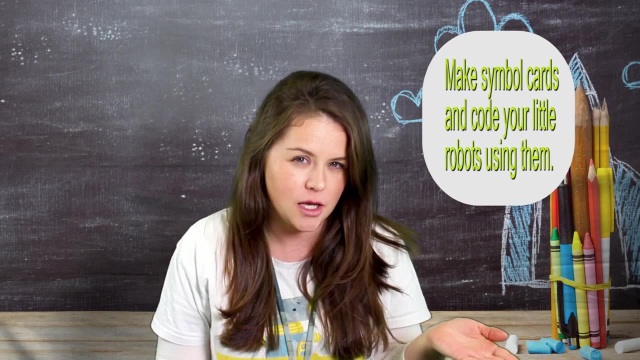 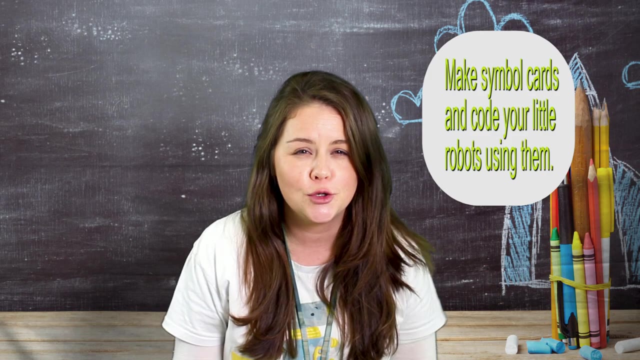 Now you're moving on to step four, four, four. This is taking the verbal coding game and turning it into a non-speaking coding game. This time, your bots are gonna stand in front of you and you are going to code them through visual symbols. 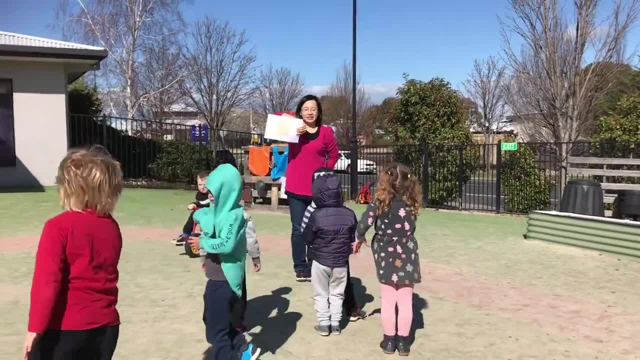 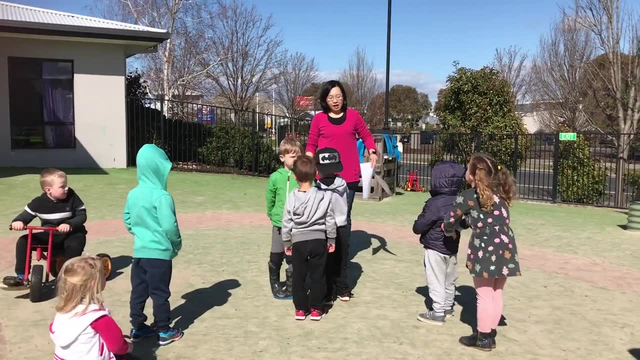 Now you can choose whatever symbols you like and maybe you can make it up together what are good actions for them to perform, And you just hold it up in front of the kids and they do the sequence for you. This is a non-talking version of the game. 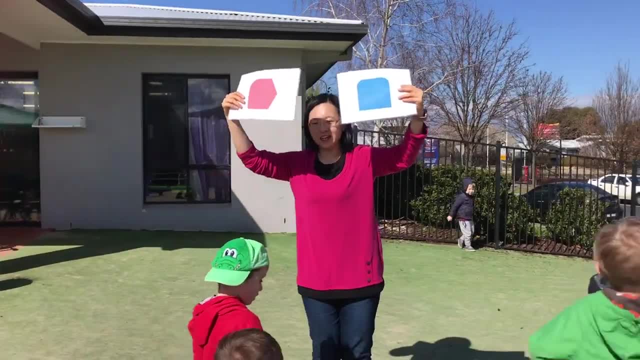 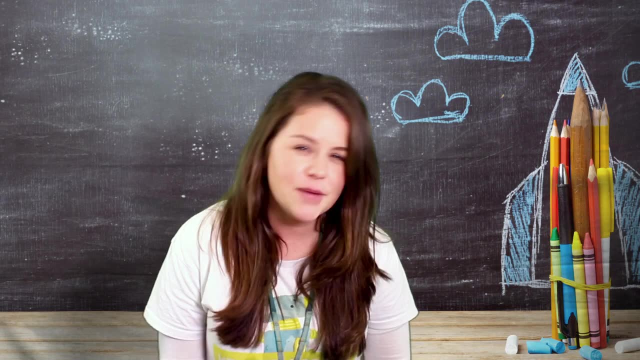 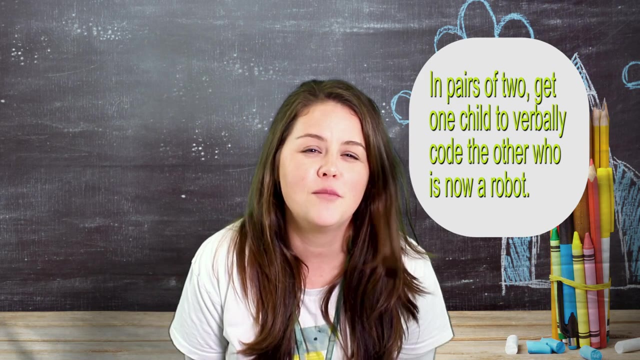 that we played before, where you code your little robots using symbol cards. So you are the coder and they follow your code. The last step I'm gonna leave you with is step five, Which is having your kids code each other. Here you're gonna pair them up into groups of two.